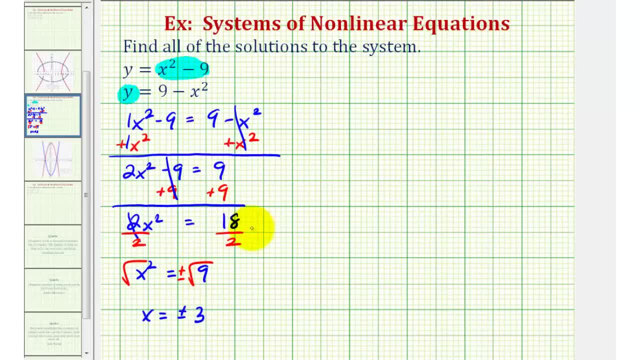 This is normally how we solve this equation. Most texts show how to solve this equation, but the real reason why we have two solutions here is because when we take the square root of x squared, it's actually equal to the absolute value of x, because the result must be positive. 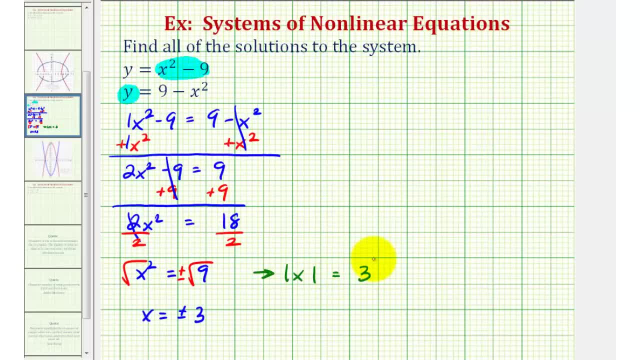 So we have: the absolute value of x equals positive three. Therefore, x can be either both positive three or negative three. So now that we know x can be either positive or negative three, we need to perform back substitution into one of the original equations. 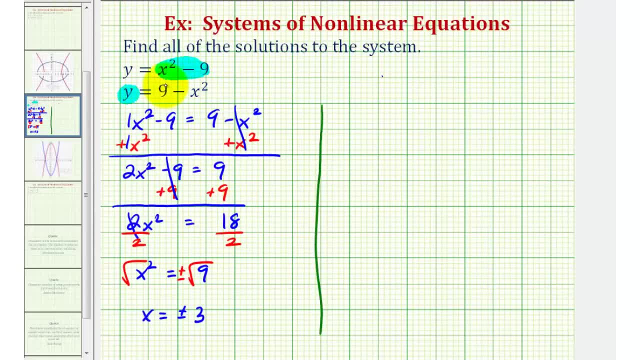 To find the corresponding y values. Let's go ahead and use the first equation, where we have y equals x squared minus nine. Let's start with x equals positive three, So we would have y equals positive three squared minus nine, So y equals nine minus nine, which is equal to zero. 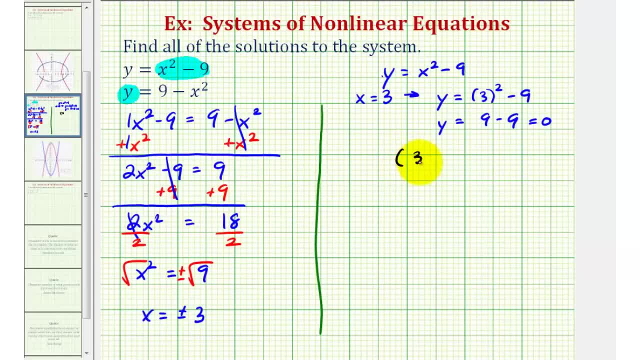 Which means when x equals positive three, y is zero. Notice, because x is squared. when x is negative three, we'll have the same corresponding y value. Let's go ahead and show it. If x equals negative three, then we have y equals negative three, squared minus nine. 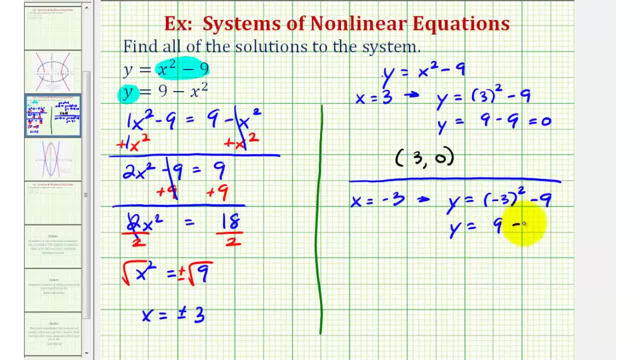 But negative three squared is still positive nine. so nine minus nine is equal to zero. Our other solution is: x equals negative three and y equals zero. So the system of nonlinear equations has two solutions, which means if you graph these two equations on the coordinate plane, 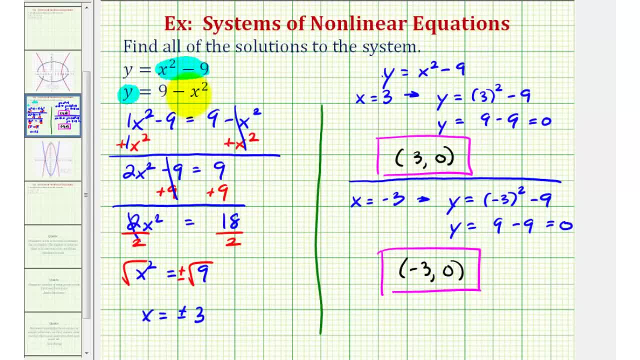 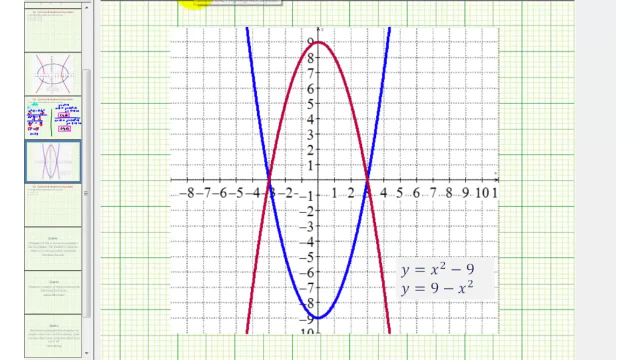 the two functions, which are parabolas, should intersect at these two points. Let's go ahead and verify that Notice: one parabola opens up and one opens down. There are two points of intersections, both on the x-axis, here and here. 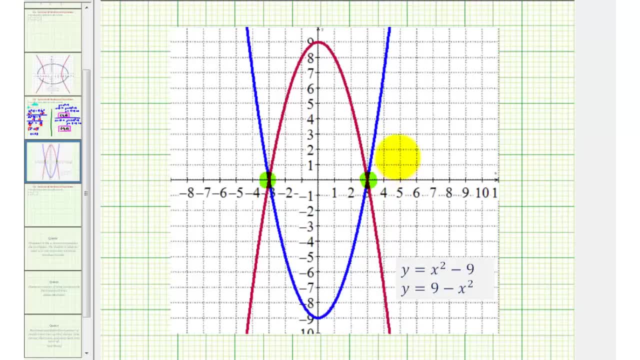 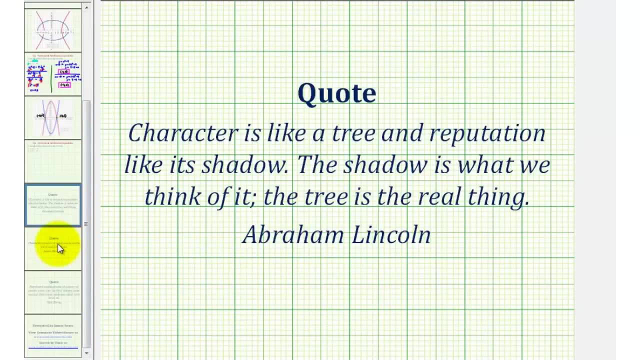 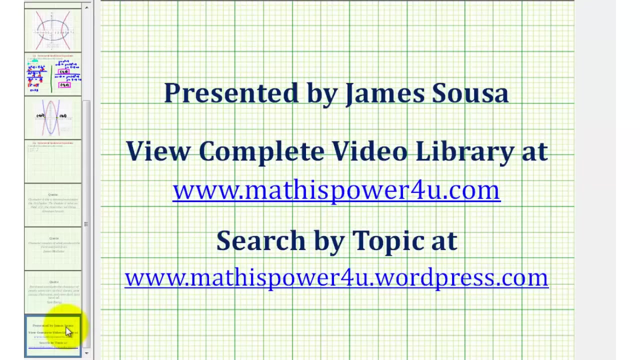 And notice, the coordinates of the points of intersection are three zero and negative three zero, which were the solutions that we found algebraically Okay. I hope you found this explanation helpful. Thank you for watching. We'll see you next time. 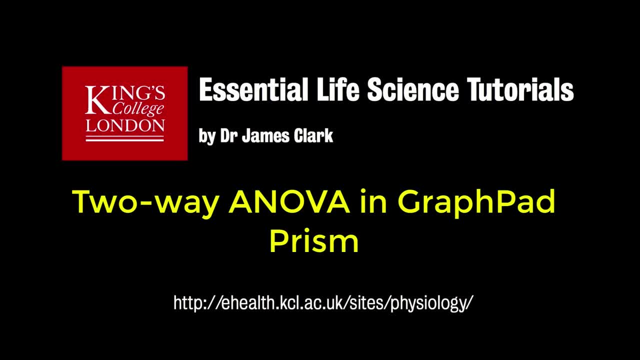 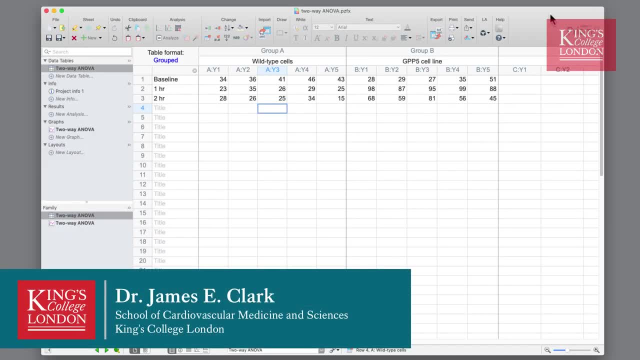 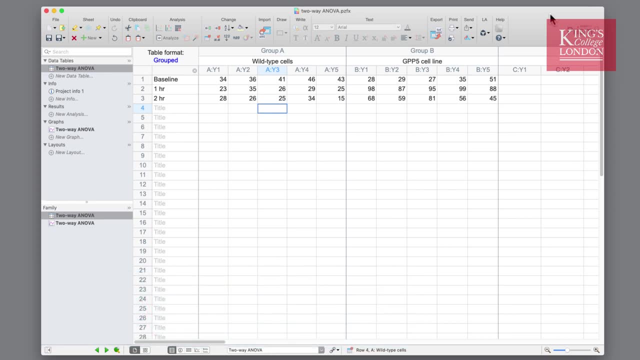 Hello, I'm James Clark from King's College London and in this short video I'm going to show you the steps required to undertake a two-way ANOVA analysis in GraphPad PRISM. You would use a two-way ANOVA rather than a one-way ANOVA when you have one measurement. 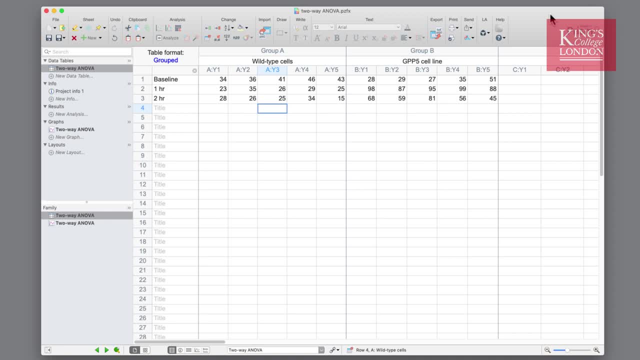 variable and two nominal variables and that each value of the nominal variable is found in combination with each value of the other nominal variable. An example of this is on the screen. We have two different cell types: wild type in group A and our GPP5 genetically. 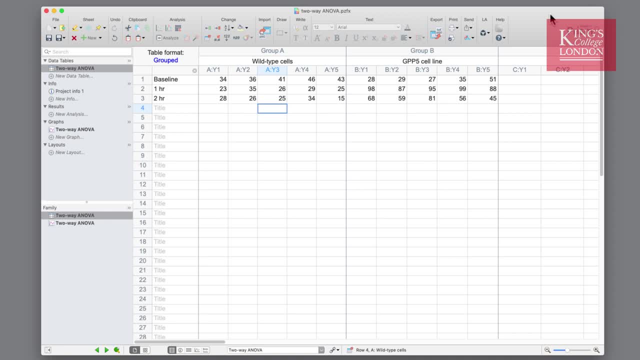 modified cell line in group B and we expose them to a drug over a period of time. So in this case the measurement variable is their viability and the nominal variables are genotype and time. This tests three null hypotheses. It tests that the mean of the measurement variable 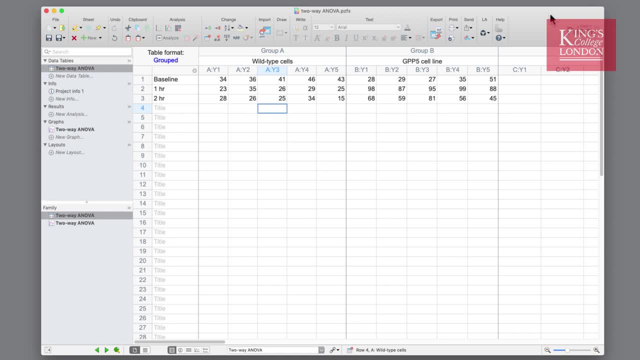 are equal for different values of the first nominal variable, in this case our genetic cell type, and that the means are equal for different values of the second nominal variable. In other words, the means are the same over time. It also tests that there is no interaction. The effects of one nominal variable don't.